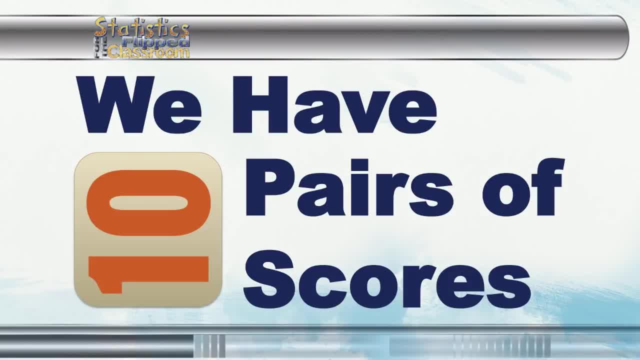 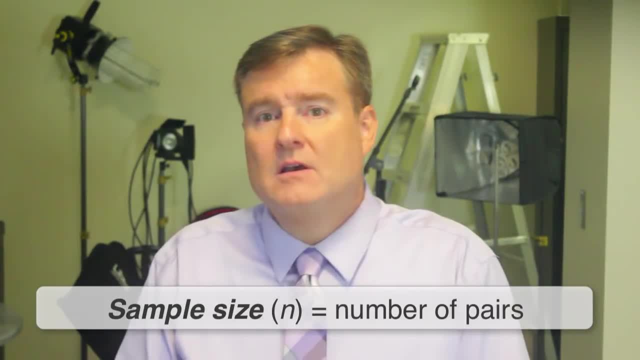 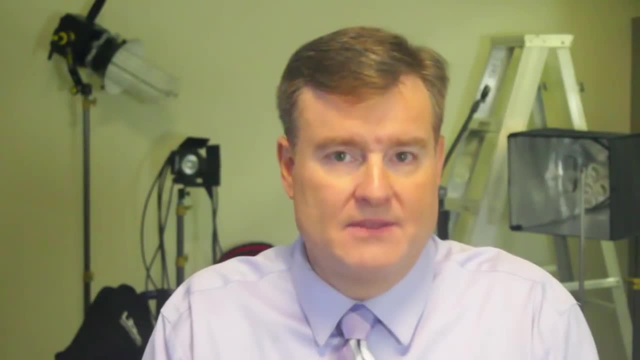 stays together. We have 10 pairs of scores. Our sample size is 10.. Each pair counts as one case, So remember that we have two people without height and weight scores. They are not going to be included in this analysis. In fact, SPSS will simply ignore those cases with missing values. 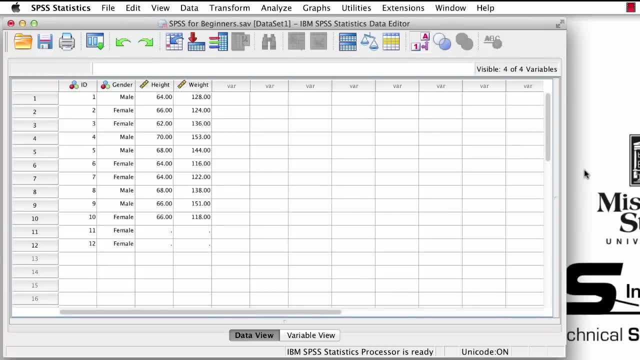 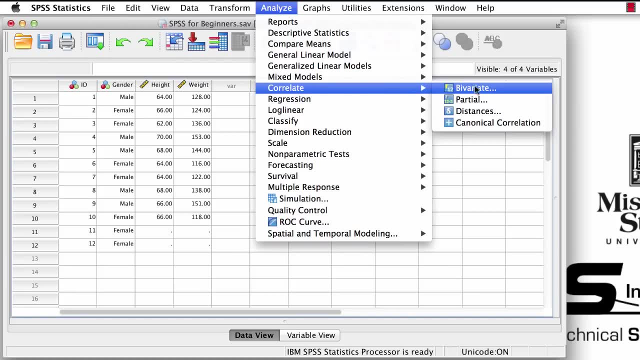 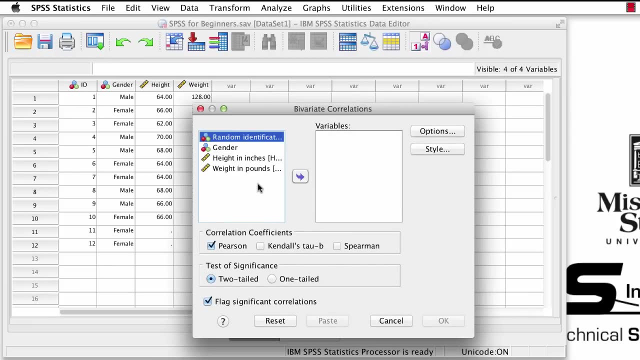 So let's do a correlation, Go to Analyze, Correlate. Now Pearson's R correlates two variables, so choose Bivariate. As before, all of our variables are here on the left. The two that we want to correlate are height and weight. 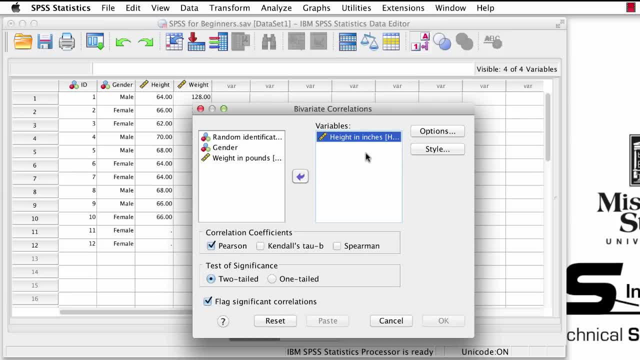 So we need at least two variables. When you move over the first, the OK is still not available until you move over the second. Now we could add additional variables, but each would be correlated, only two at a time. We have some additional options here as well. We could calculate. 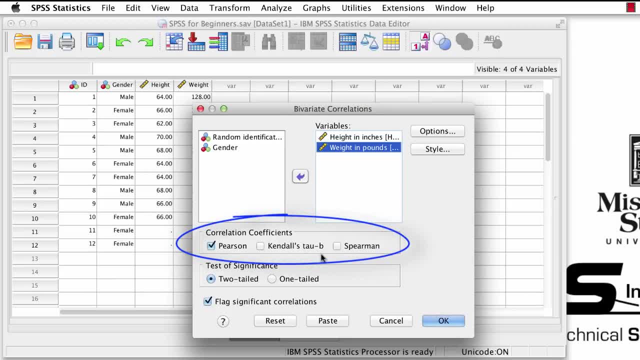 Kendall's tau or Spearman's rho if we had different data. But for now let's just stick with Pearson's R. SPSS assumes that we want two-tailed significance tests and that we want to flag significant correlations. But we haven't talked about significance tests yet. So for now, 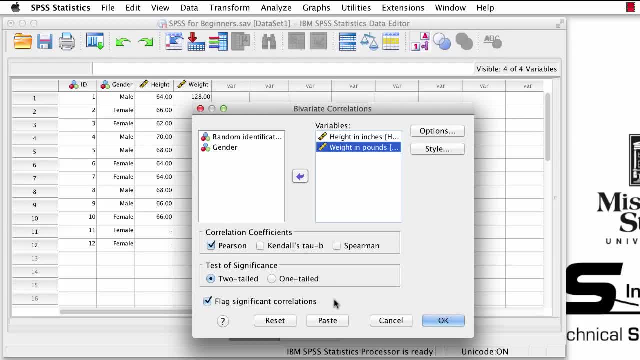 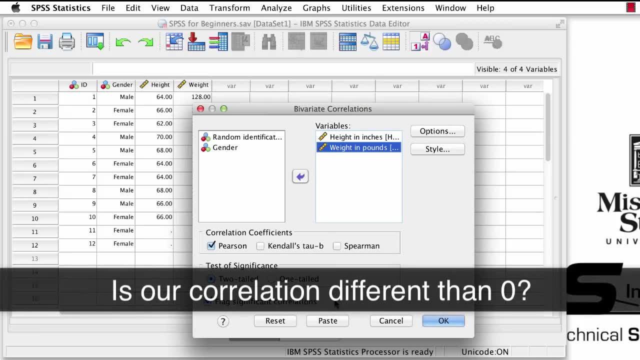 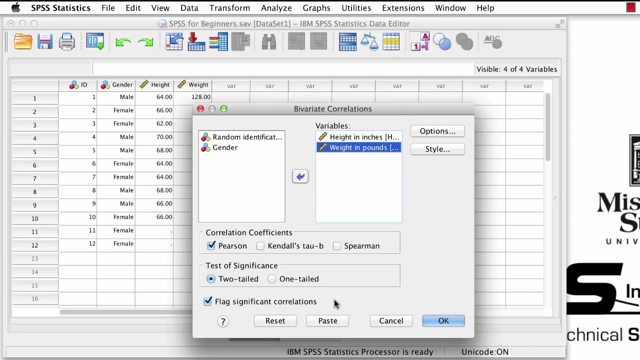 just know that significance tests tell us something important about the variables. In this case, our correlation is statistically significantly different than zero. If it is, SPSS will flag it. All of the default settings are just the way we want them, So click OK to run the analysis. 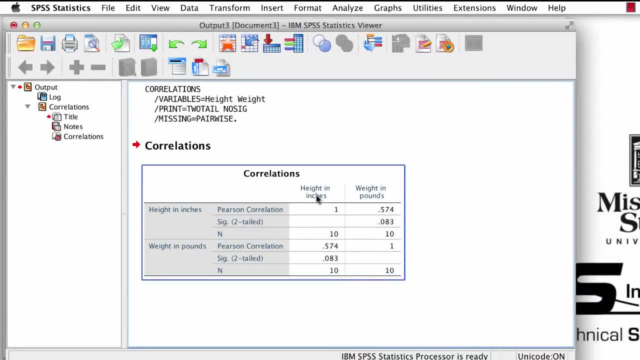 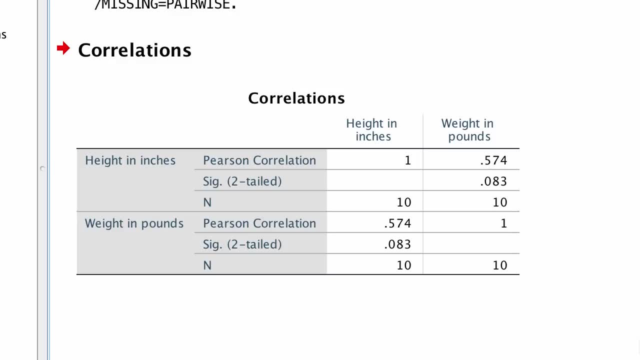 The box that we see is called a correlation matrix. The correlation matrix shows the correlation coefficient for every combination of variables. So we have two rows, one for height, one for weight, and we have two columns, One for height, one for weight- Where each row and column 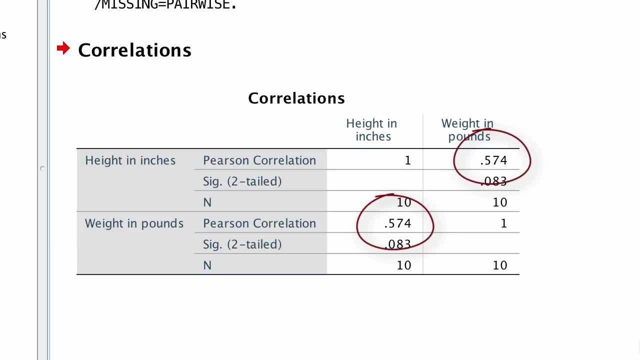 intersect, we see the correlation coefficient between those two variables. So in this quadrant of the matrix we see the correlation coefficient between height and itself. No surprise, it's one. It's a perfect correlation. We see another perfect correlation down here on the lower right. 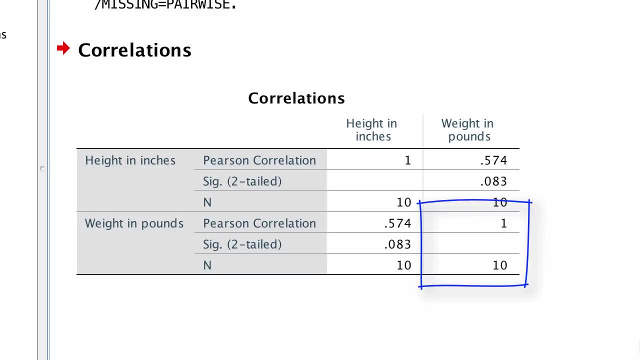 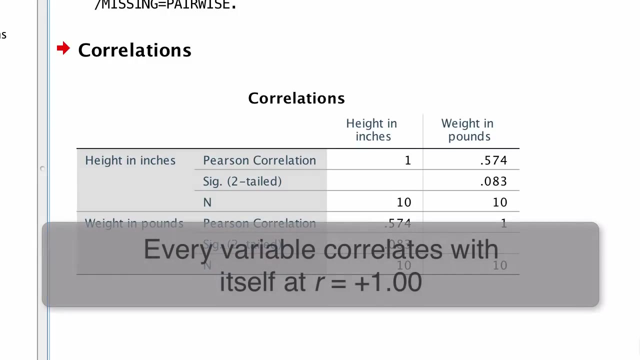 which is the correlation between weight and itself. SPSS will compare every combination of variables, including each variable and itself. Now these correlations are not very interesting because we already know that every variable will always correlate with itself at a positive one, no matter the variable The interesting. 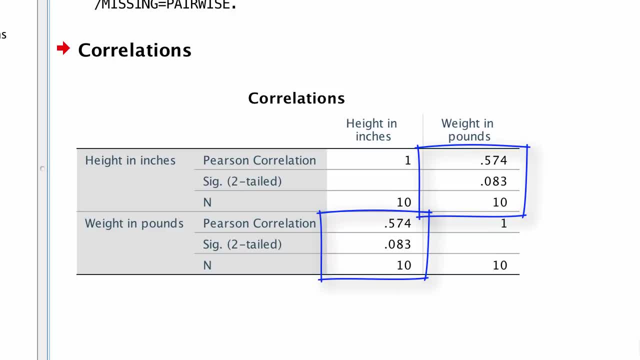 correlations are in these off diagonals. The top left box is the correlation coefficient. It will always be between positive one and negative one. Below that is the significance level. Significance levels smaller than 0.05 are statistically significant. Below that is the n or the sample size. 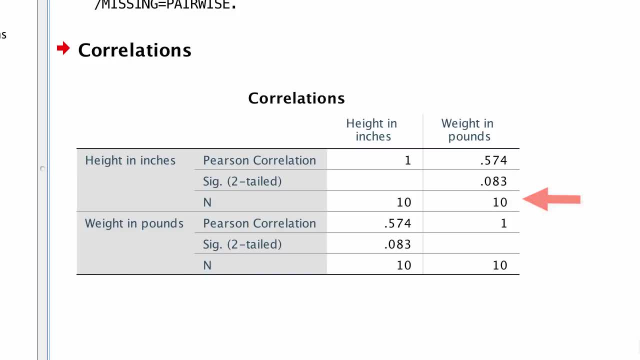 which is our 10 pairs of scores. So let's look at this coefficient. Notice that the off diagonal correlations are the same, because height correlates with weight, exactly the same as weight correlates with height. In this case it's a 0.574,. 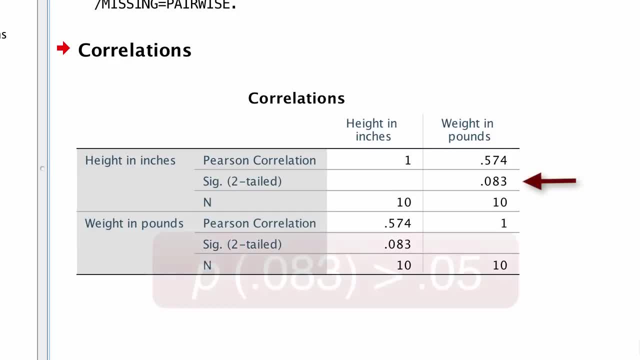 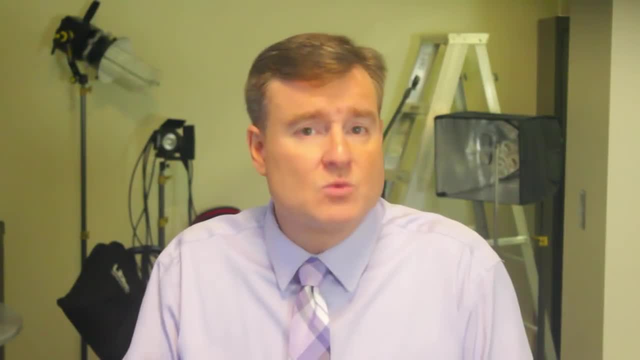 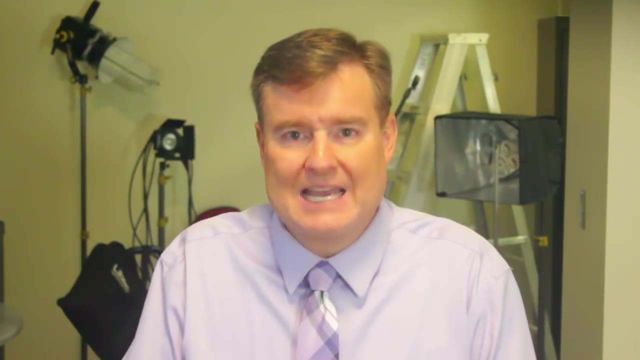 which is pretty strong but not significant because the sample size of 10 is pretty small. You are always more likely to find significance with larger sample sizes. If this correlation was significant, we would see some asterisks next to the coefficient. So, as I mentioned, 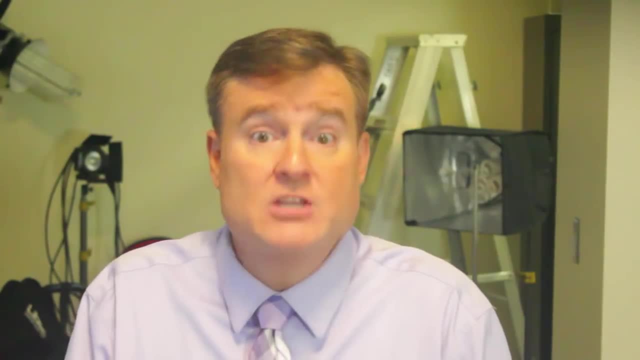 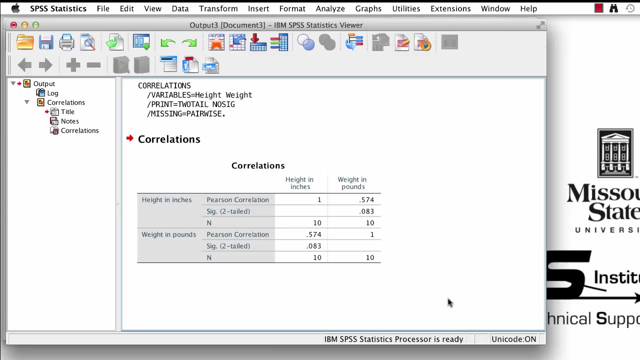 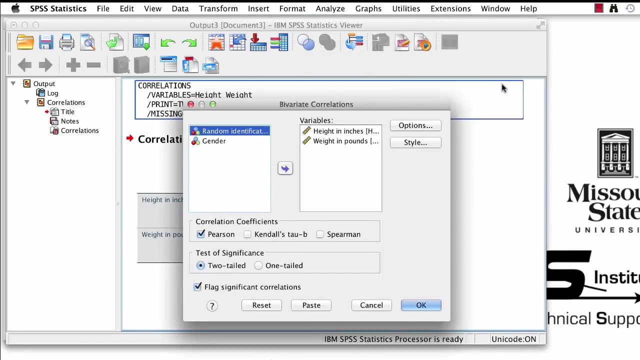 you can correlate more than two variables at a time, and you could even use correlation with nominal variables, as long as it only has two levels. In fact, let me show you. Go to analyze correlate bivariate. All we're going to do is throw in a third variable, gender. 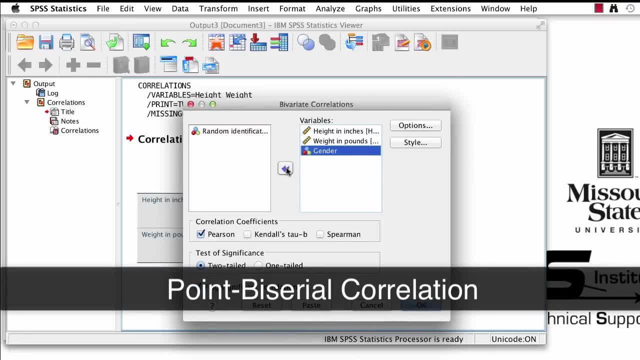 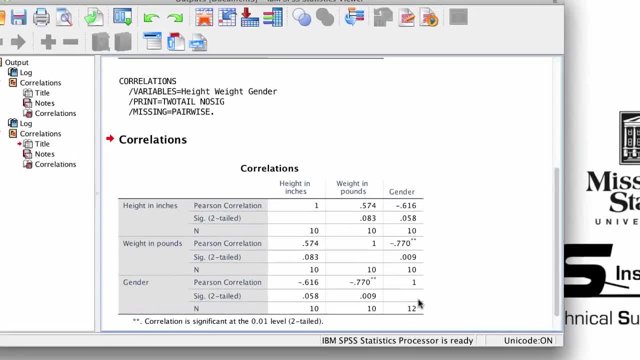 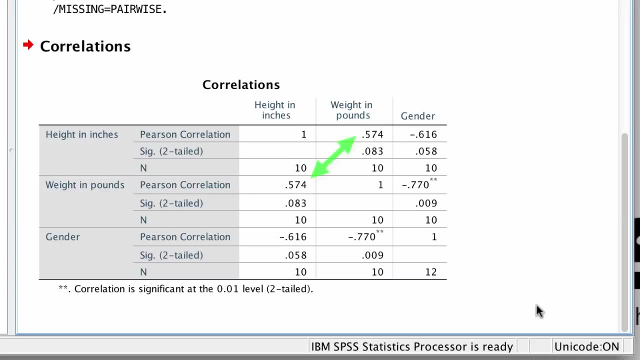 and this is actually called a point-biserial correlation. More on all of that later. For now, just click OK, We get another correlation matrix, But this time it's bigger. It has three rows and three columns. The correlations between height and weight are exactly the same as before. 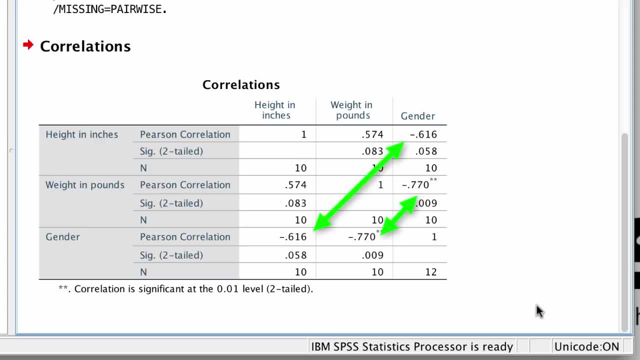 but we also have correlations with gender, Because the correlations are negative: as one variable goes up, the other goes down. Remember that we coded males as 1, females as 2, so the 1 is smaller. We see this negative correlation: The smaller numbers are associated. 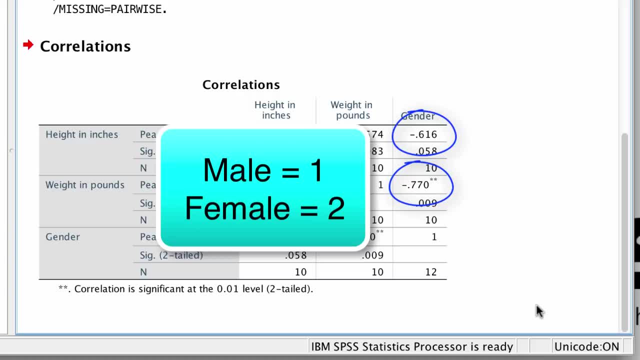 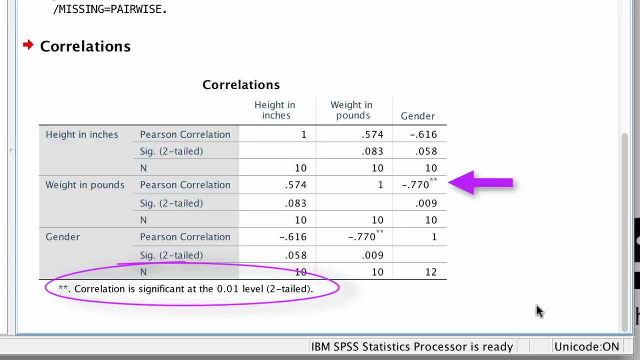 with larger values. So basically, the males were taller and weighed more, And here we also see a significant correlation that has been flagged. The biserial correlation between weight and gender has two asterisks. So what does that mean? We can see that this correlation is significant at the 0.01 level. 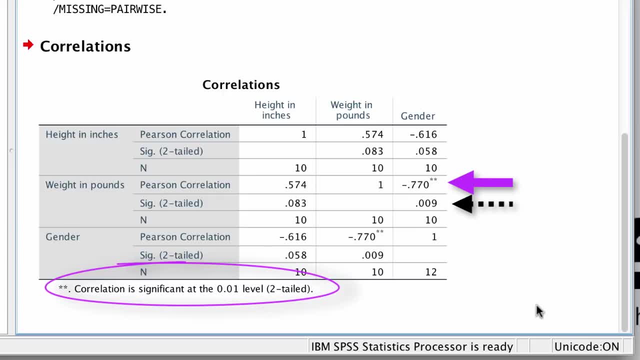 In fact, the p-value was 0.009.. So there is a significant correlation at the 0.01 level. In fact, the p-value was 0.009.. So there is a significant correlation at the 0.01 level. 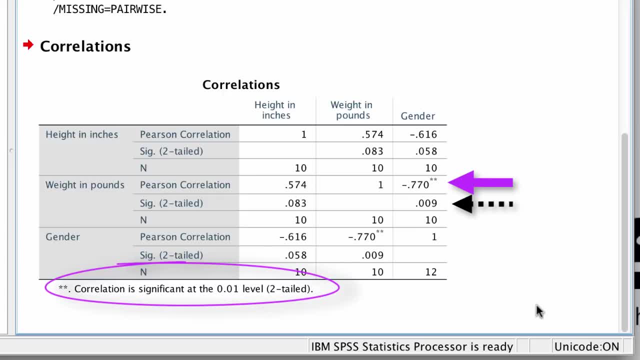 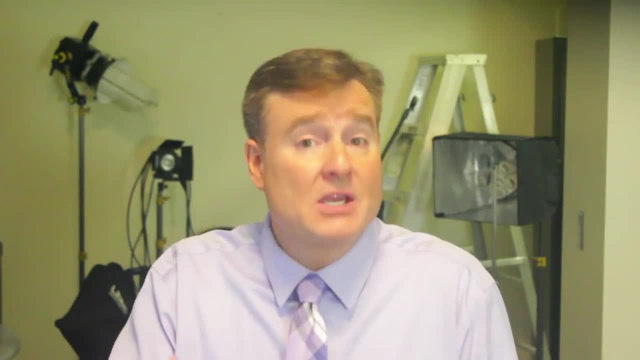 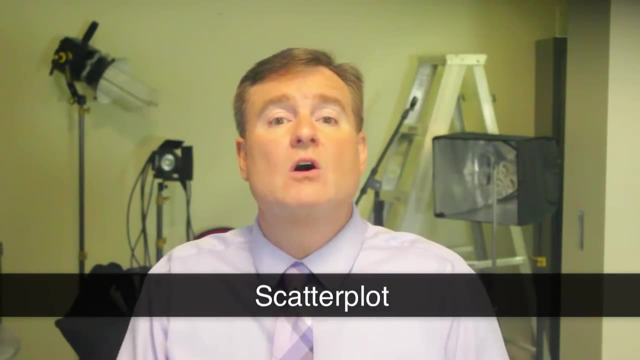 So there is a statistically significant relationship between weight and gender. So there's one more thing that I want to show you with correlations, and that is how to make a picture of them. The picture is called a scatterplot, and it is created using a new tool called the Chart Builder. 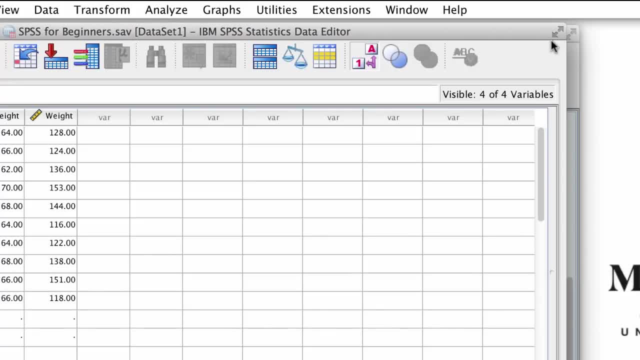 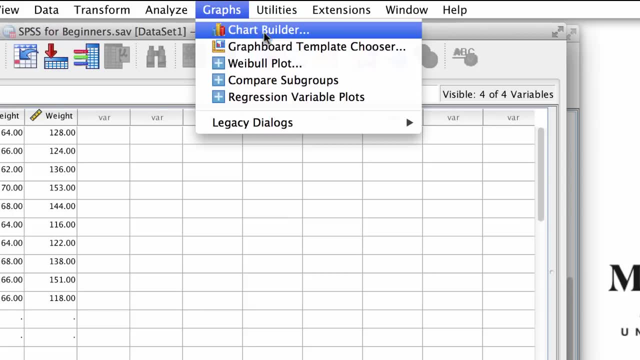 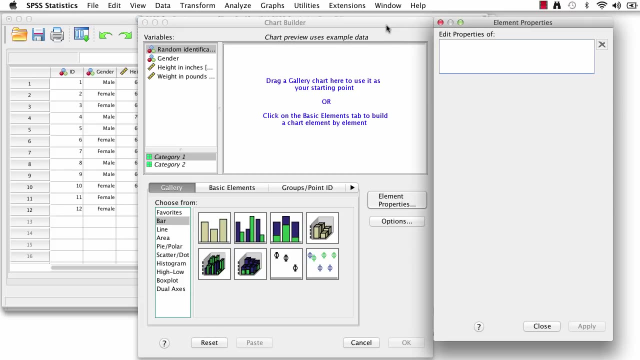 And here is how we do it. Instead of the Analyze menu, we're going to use the Graphs menu, So go to Graphs Chart Builder. We will learn more about the Chart Builder later, when we learn about graphing. For now, let's just have some fun and make a scatterplot. 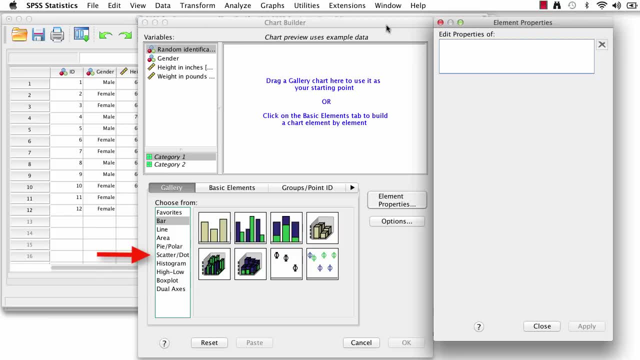 Start by clicking on the word scatter dot in the gallery. Now we see our eight options. If you hover your cursor above them, SPSS will tell you what they are. We want this first option: Simple Scatter Click and drag it into the blank area known as the Canvas. 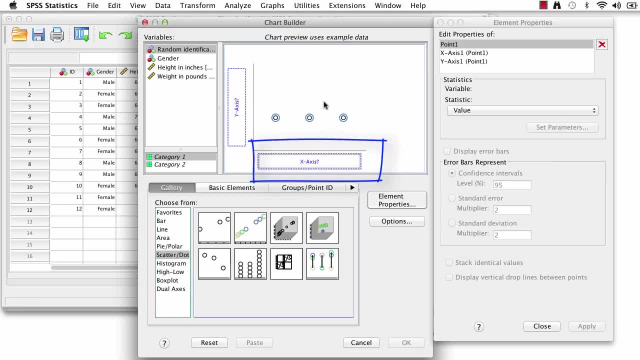 You will see that we now have two drop zones: one for the X-axis and one for the Y-axis. So let's use Height to predict Weight, Drag Height to the X-axis drop zone and Weight to the Y-axis drop zone, And that is all you have to do. Click OK. 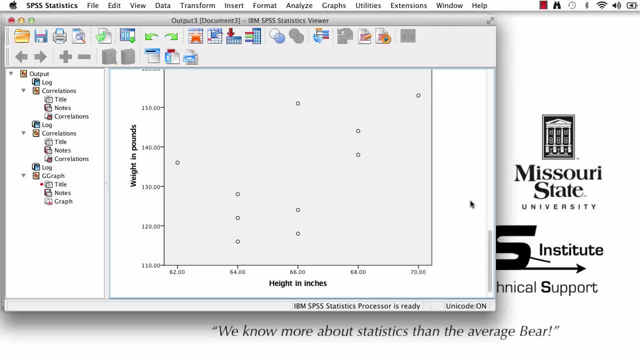 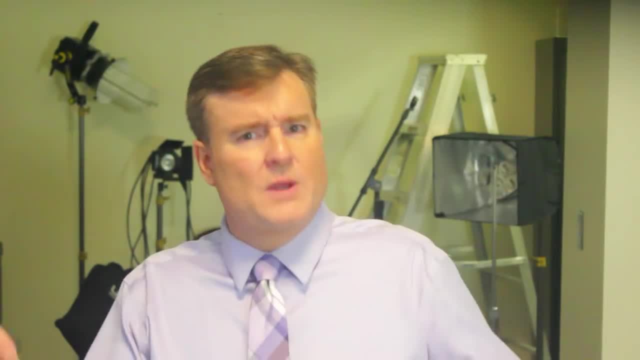 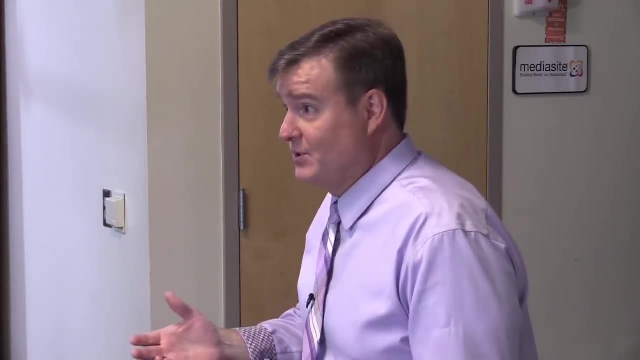 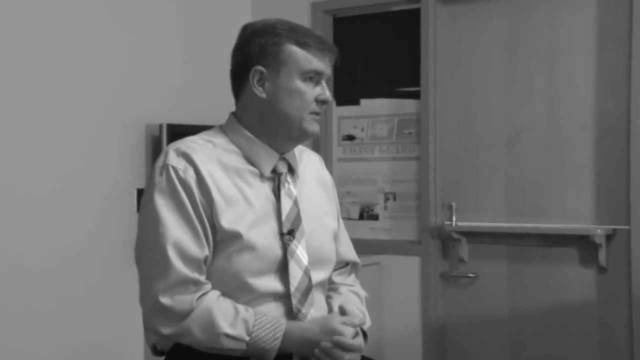 And there is our scatterplot of all ten of the pairs of scores. There is much more that we could do with correlation. So, for instance, we could format the scatterplot in APA style. We could do other types of correlations. We could even use some variables to predict other variables, using a technique called regression.